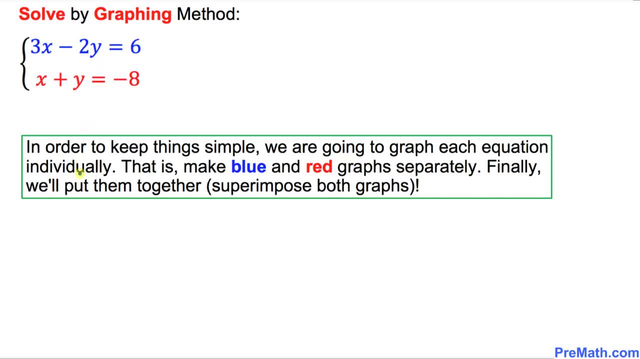 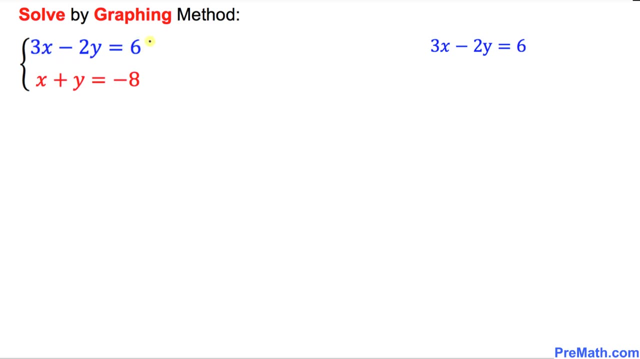 going to graph each of these equations individually. That means we are going to make red and blue graphs separately. Finally, we will put them together. That means we are going to superimpose them. So in our very first step, we are going to look at the very first equation, the top one. 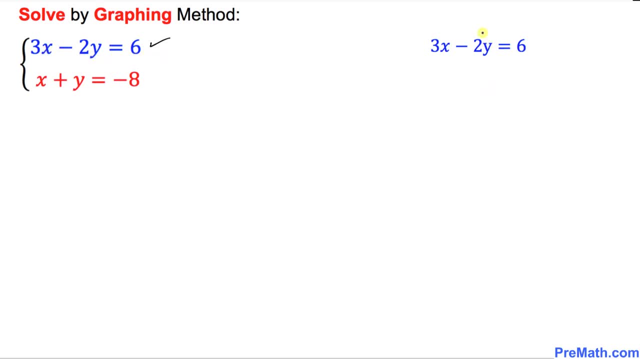 3x minus 2y equal to 6.. I just put it down over here And let's go ahead and solve for x and y. Let me show you an easy way of doing this one. I am going to put down x and y chart. 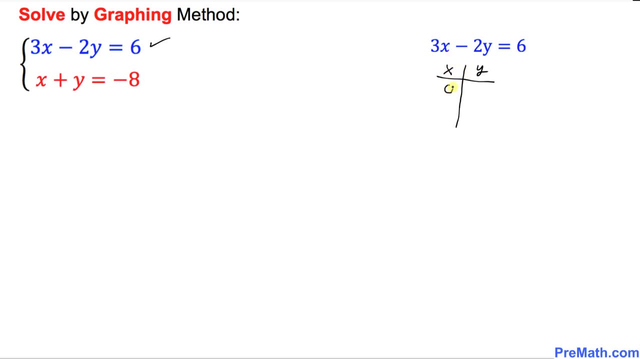 What I am going to do is That's what we had in our strategy- Put x equal to 0 and solve for y. That means, wherever your x is going to be, you just put down 0. If you plug it in this 0, this is going to. 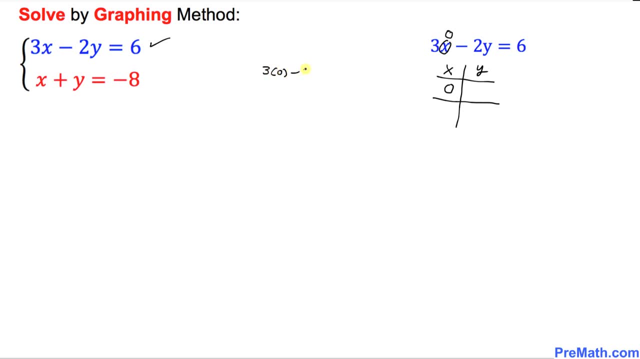 become 3 times 0 minus 2 times y, equal to 6.. 3 times 0 is 0 minus 2y, equal to 6.. So we got negative 2y equal to 0.. And now we are going to solve for the last one. We are going to put down x and y and 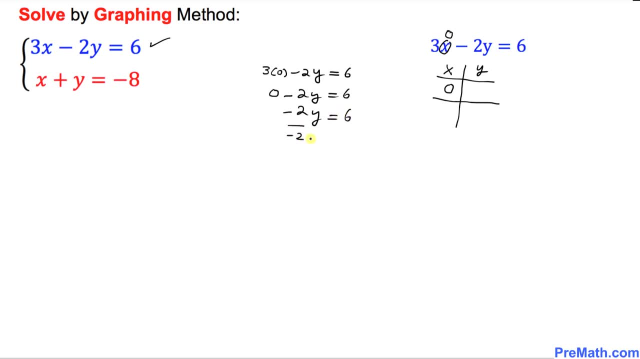 we are going to solve for y. This is going to be just the same thing, Just a little bit more easy. We are going to apply this to this equation. then We are going to get a bit of our 6. You divide both sides by negative 2. So y turns out to be negative. 3. So that means if x equal to 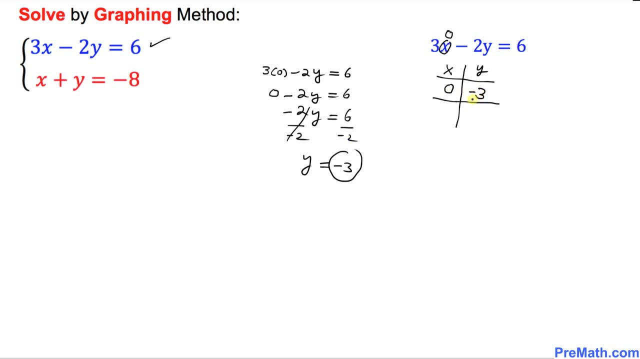 0, y is going to be negative 3. And in our next step, this time I am going to put y equal to 0 and we are going to find x value. That means, wherever you see y, this becomes 0. So let's. 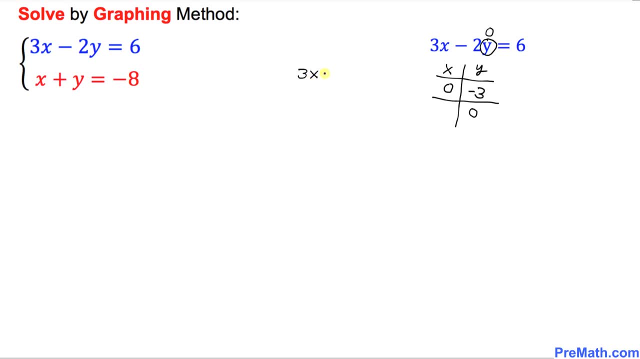 simplify that one. So we got 3x minus 2 times 0, equal to 6.. So 3x 2 times 0 is 0, equal to 6.. 3x minus 0, equal to 3x, equal to 6.. Divide both sides by 3.. So x turns out to be 2.. So that means when: 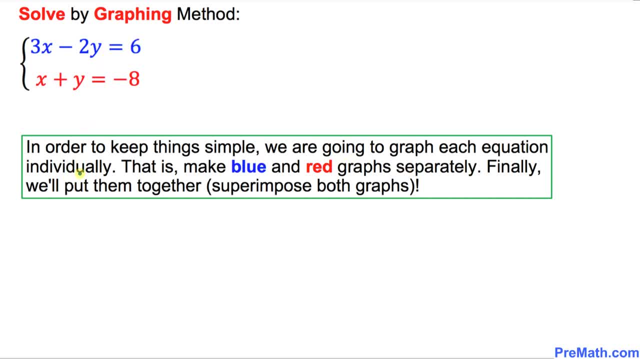 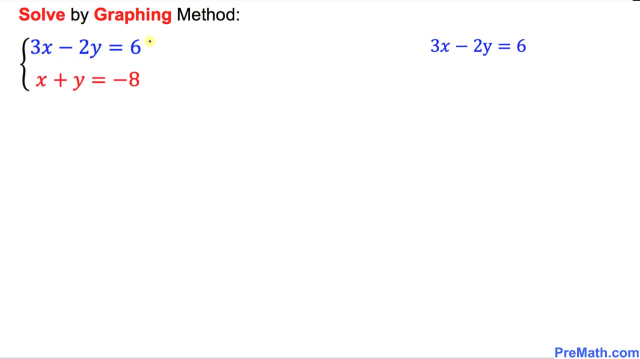 going to graph each of these equations individually. That means we are going to make red and blue graphs separately. Finally, we will put them together. That means we are going to superimpose them. So in our very first step, we are going to look at the very first equation, the top one. 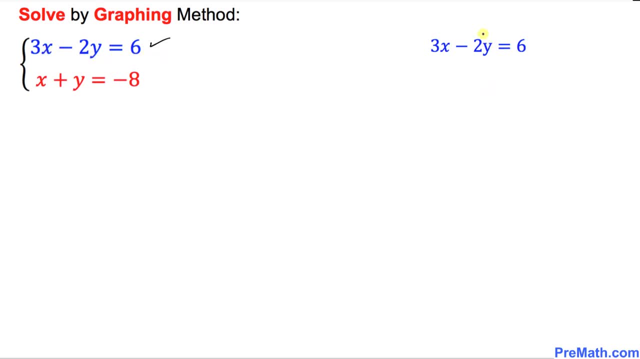 three x minus two y equal to six. I just put it down over here And let's go ahead and solve for x and y. Let me show you an easy way of doing this one. I am going to put down x and y chart. 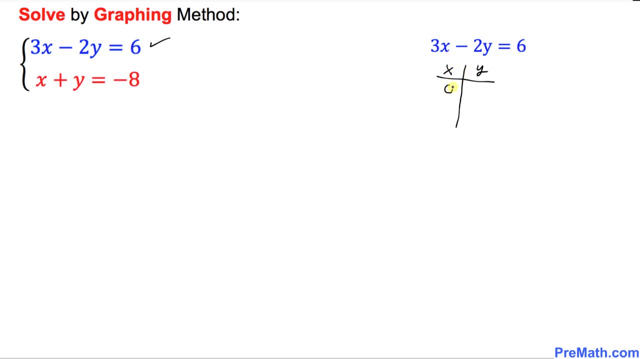 What I am going to do is- here is going to be our strategy: put x equal to 0 and solve for y. that means, wherever your x is going to be, you just put down 0. if you plug it in this 0, this is going to become 3 times 0 minus 2 times y, equal to 6. 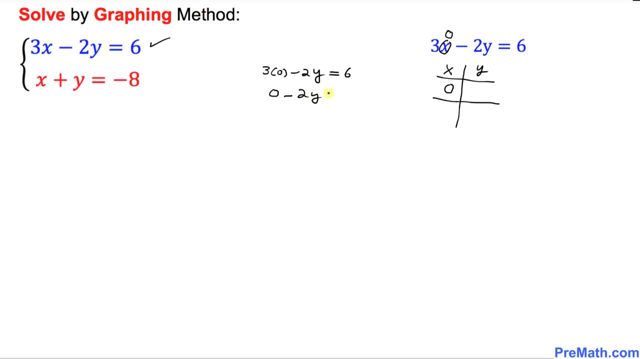 3 times 0 is 0 minus 2, y equal to 6. so we got negative 2, y equal to 6. you divide both sides by negative 2, so y turns out to be negative 3. so that means if x equal to 0, y is going to be. 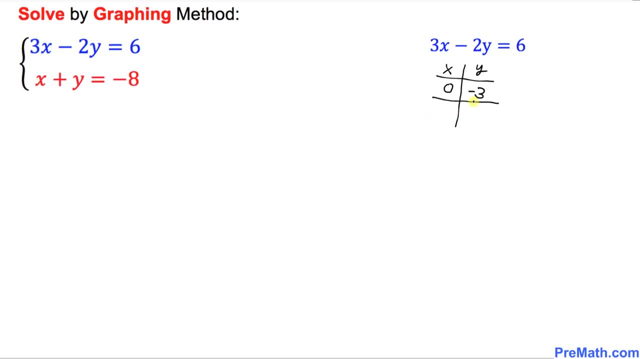 negative 3 and in our next step, this time I'm going to put y equal to 0 and we are going to find x value. that means wherever you see y, this becomes 0. so let's simplify that one. so we got 3x minus 2 times 0 equal to 6. so 3x 2 times 0 is 0 equal to 6, 3x. 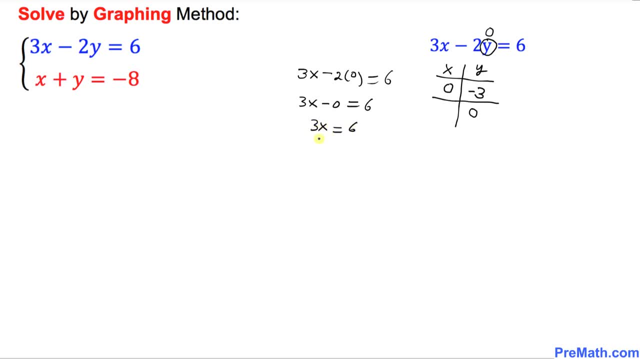 minus 0 equal to 3x equal to 6. divide both side by 3, so x turns out to be 2. so that means, when x equal to, when y equal to 0, x is going to be 2. so thus we got 0 comma negative 3. the other one is: 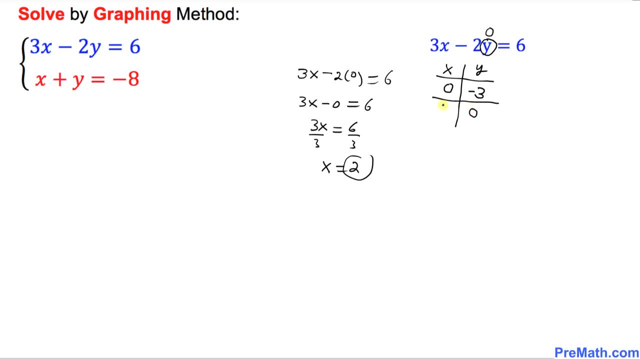 x equal to when y equal to 0,, x is going to be 2.. So thus we got 0 comma negative 3.. The other one is 2 comma 0.. I am going to put it down right up here: One of the point is 0 negative 3.. The other one is 2 comma 0. 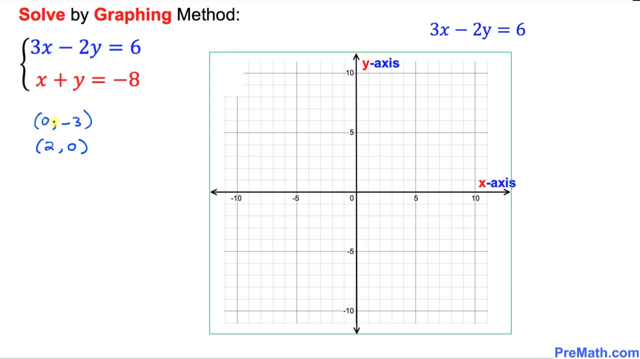 And now let's go ahead and plot these two points that we figured out. The first one is 0, negative 3.. So where is going to be 0, negative 3 is going to be right up here, isn't it? So? 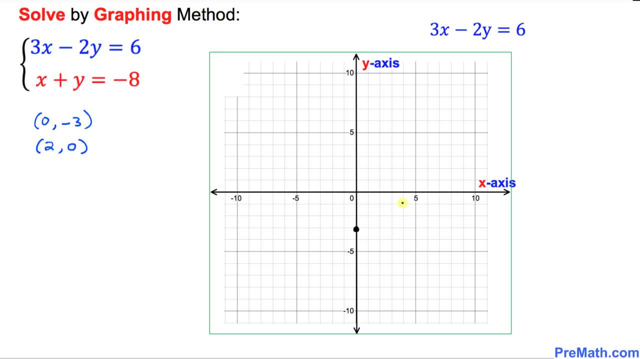 this is 0, negative 3.. The other one is 2, 0.. So 2, 0 is going to be this one right now. As you can see that this one is the point is on x axis. No wonder we call it x intercept. 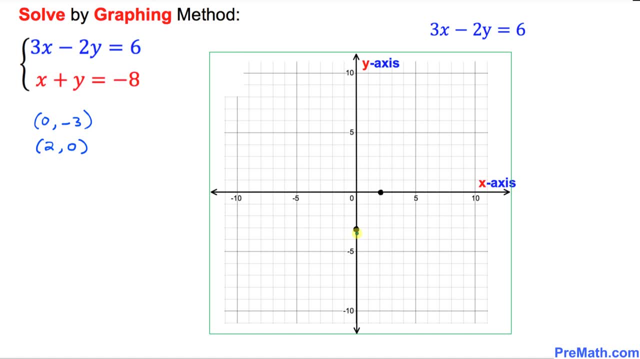 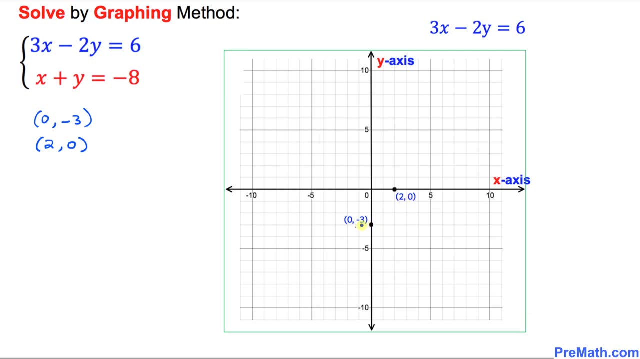 And this point is on y axis. we call it y intercept. And here I have nicely plotted these points and I give them a name: 2, 0 and 0, negative 3.. The next thing, what we're going to do, is to we can construct a straight line by connecting these two points. And here is the. 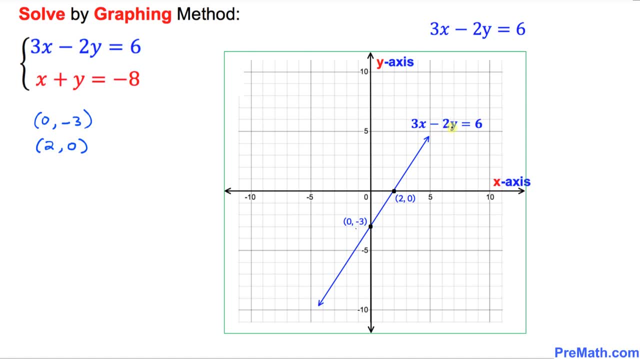 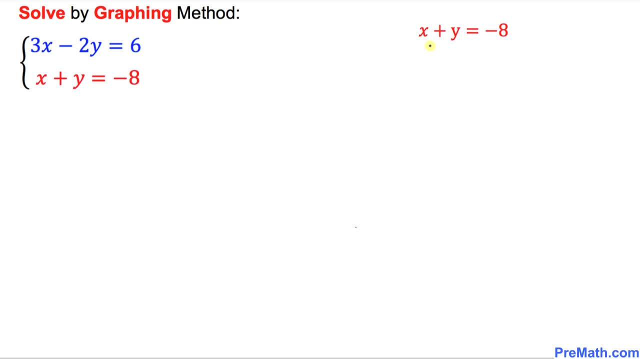 graph for our blue equation: 3x minus 2y equal to 6.. Now let's focus on our red equation, the bottom one, and we want to graph this thing. So, once again, the very first step is we are going to create a t chart. I am going to put down: 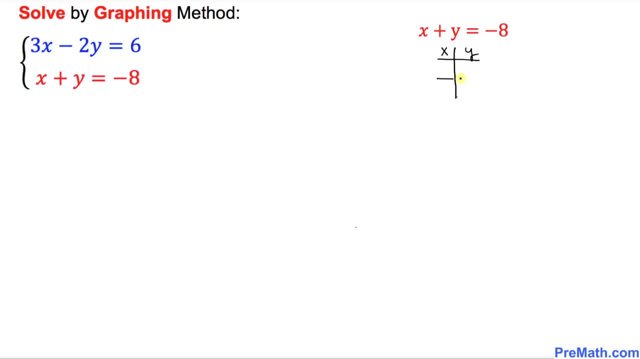 x right up here. y Same thing we're going to do once again. First, we're going to put x value 0 and figure out y value. So wherever you see x, this becomes 0.. So that means let's simplify. 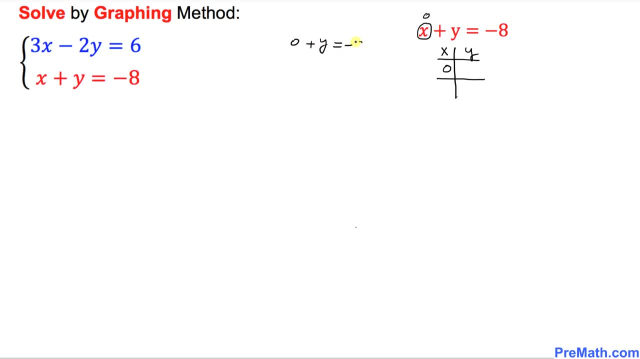 So 0 plus y equals to negative 8.. 0 plus y is same as negative 8. So that means y value turns out to be negative 8. That means, if x is 0, y is negative 8.. Now in the next step we are going. 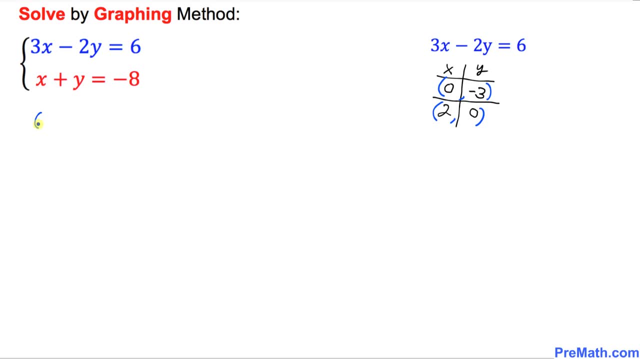 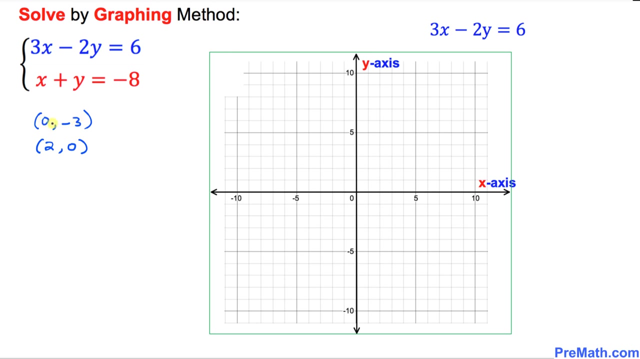 2 comma 0. I'm going to put it down right up here. our one of the point is 0 negative three. the other one is two comma zero. and now let's go ahead and plot these two points that we figured out. the first one is zero, uh, zero negative three. so where is going to? 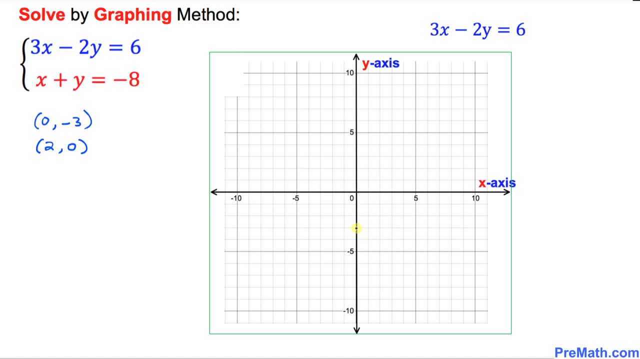 be zero negative three is going to be right up here, isn't it? so this is zero negative three. the other one is two zero. so two zero is going to be this one right now. as you can see that this one is, the point is on x-axis- no wonder we call it x intercept and this point is on y-axis. we call it. 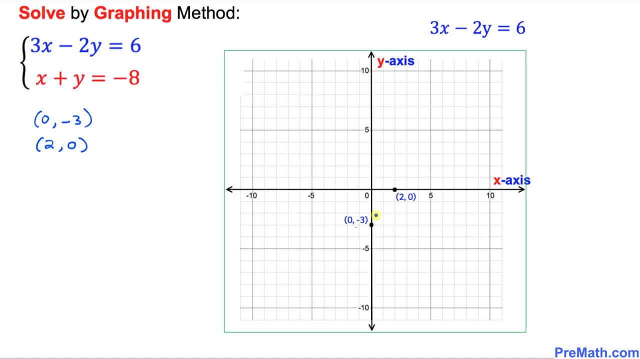 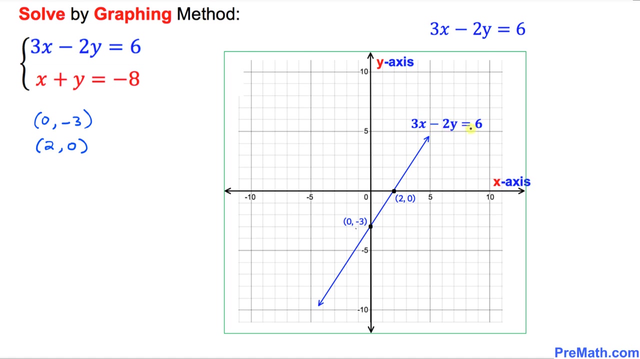 y, intercept. and here i have nicely plotted these points and i give them a name: two zero and zero negative. 3, 2, three. the next thing, what we're going to do is to: we can construct a straight line by connecting these two points. and here is the graph for our blue equation: 3x minus 2y, equal to 6. now let's: 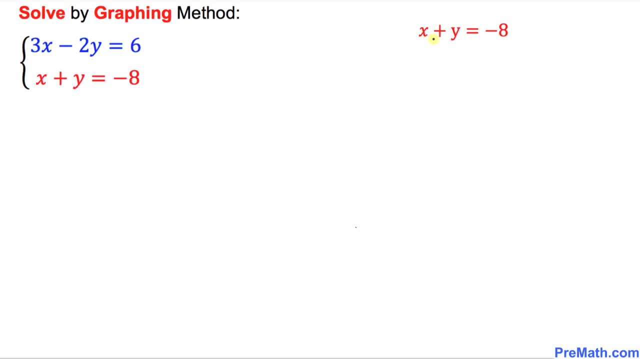 focus on our red equation, the bottom one, and we want to graph this thing. so, once again, the very first step is we are going to create a t chart. i am going to put down x, right up here. y same thing we're going to do once again. first, we're going to put x value zero and figure out y value. so 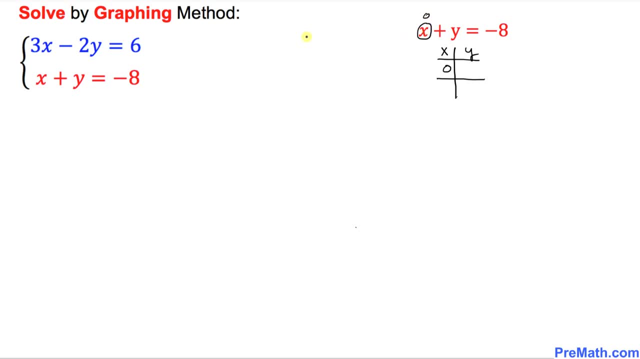 wherever you see x, this becomes zero. so that means: let's simplify. so zero plus y equals to negative eight, zero plus y same as negative 8. So that means y value turns out to be negative 8. That means, if x is 0, y is negative 8.. Now in. 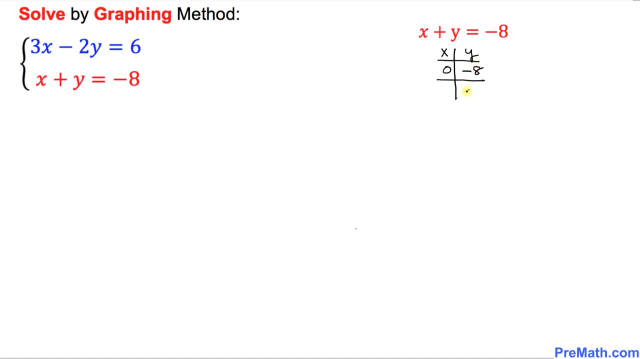 the next step we are going to plug it in y equal to 0 and see what x value is going to be. That means this time y is 0.. Let's simplify: x plus 0 equal to negative 8.. So x plus 0 is same as x. 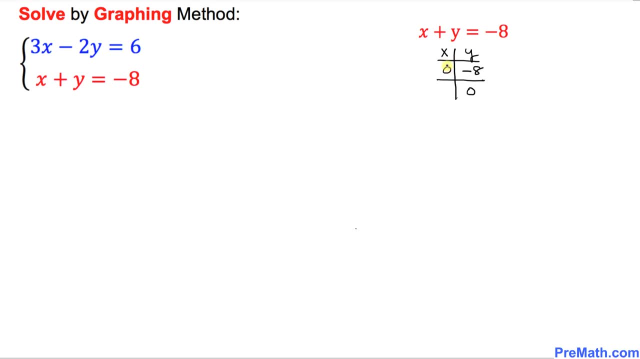 to plug it in y equal to 0 and see what x value is going to be. That means this time y is 0.. Let's plug it in y equal to negative 8.. So x plus 0 is same as x equal to negative 8. So that means y value. 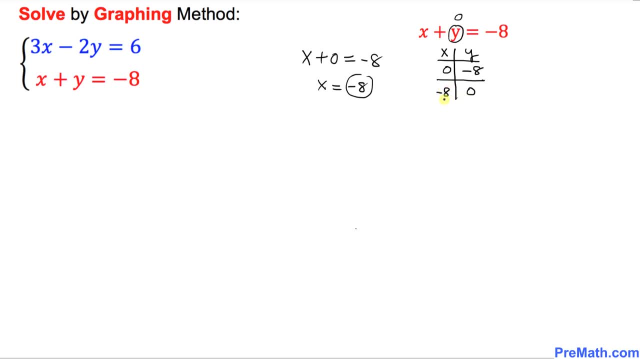 turns x value turns out to be negative 8.. So that's our two points. turns out to be a 0 comma negative 8.. The other one is negative 8 comma 0.. Let me put them down over here. So the first one: 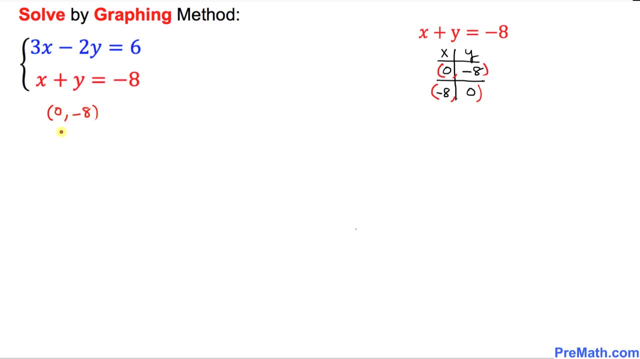 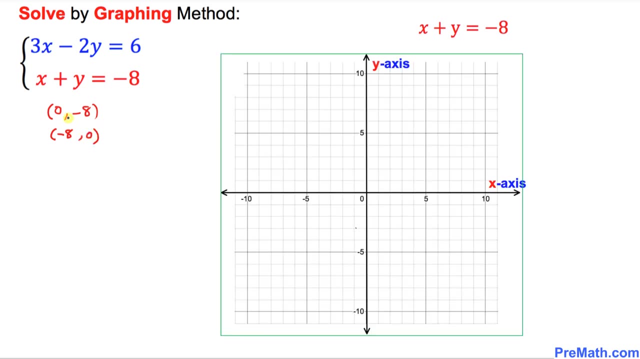 is 0 comma negative 8.. And the other one is negative 8 comma 0.. So that means y value turns out to be negative 8 comma 0.. And in this next step we are going to plot these two points on this. 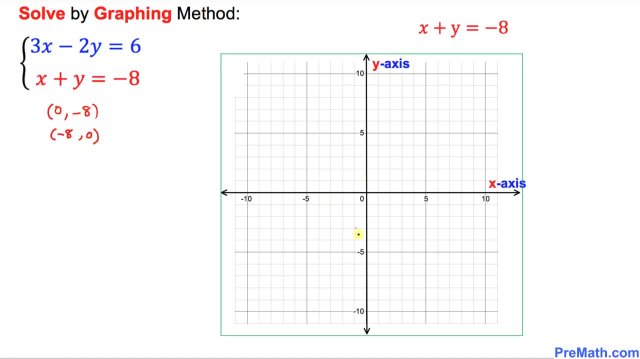 Cartesian plane. So first one is 0, negative 8.. So 0 comma negative 8 is going to be right up here, And the other one is negative 8.. 0 is going to be right up here, the point. So once again, this point is on x-axis, We're going to call it x-intercept And this point on y-axis. 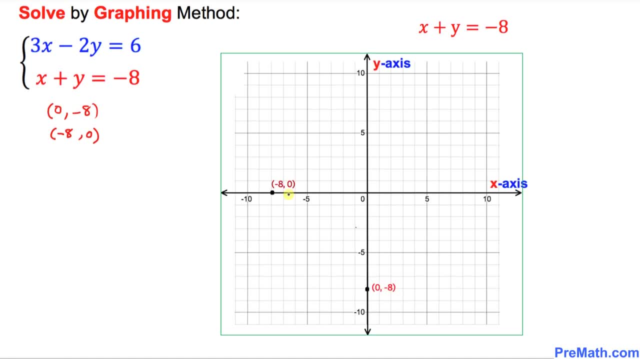 is called y-intercept, And here I have nicely plotted these points and give them a name: negative 8, 0.. And this is 0 comma, negative 8.. The next step is we are going to connect these two points to get our straight line graph. 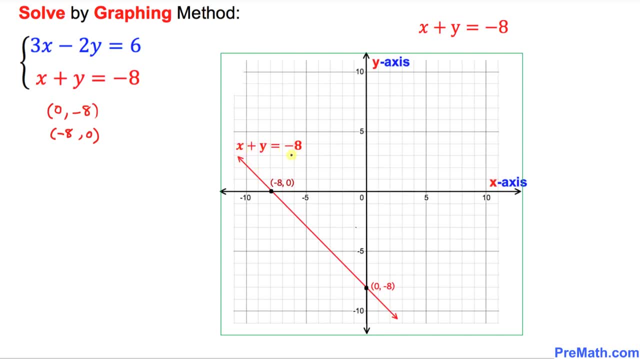 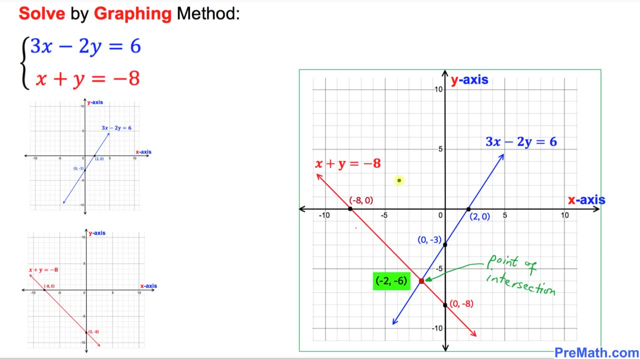 Finally, here is the graph, for x plus y equals to negative 8,, which is a straight line. And here is our final product. And on the left-hand side you see these two individual graphs And when I superimpose them, I put them together. This is the point: negative 2,, negative 6.. This is the point. 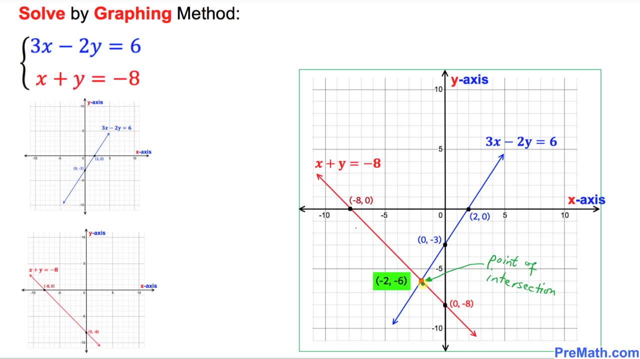 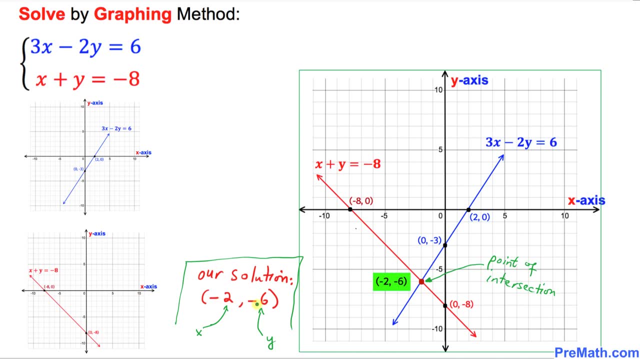 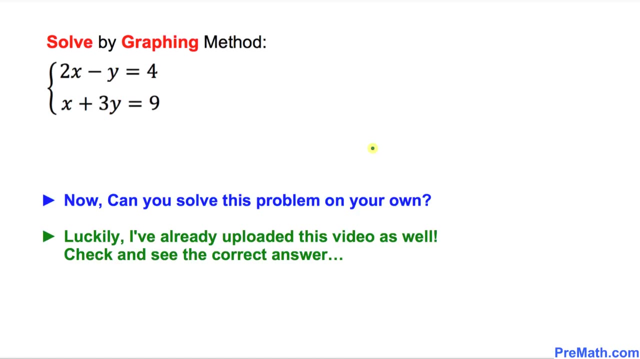 of intersection of these two lines, And that is our solution. Our solution turns out to be a negative 2 comma, negative 6.. That means x is negative 2 and y is negative 6.. And here is your assignment. Can you do this problem on your own? You can take your time, You can pause. 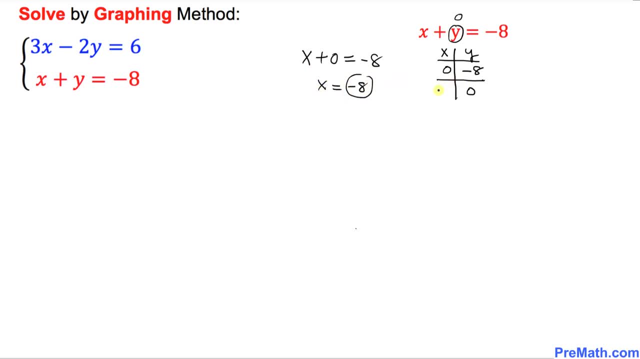 equal to negative 8.. So that means y value turns x value turns out to be negative 8.. So that's our two points turns out to be a 0 comma negative 8.. The other one is negative 8 comma 0.. Let me put. 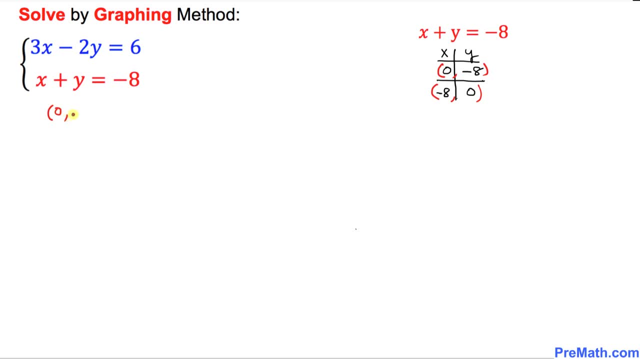 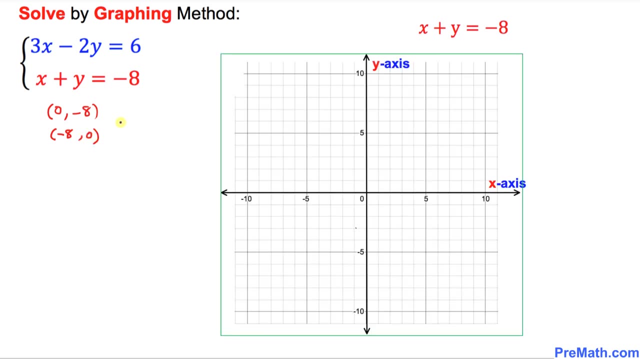 them down over here. So the first one is 0 comma negative 8 and the other one is negative 8 comma 0. And in this next step we are going to plot these two points on this Cartesian plane. So first one is 0, negative 8.. So 0 comma negative. 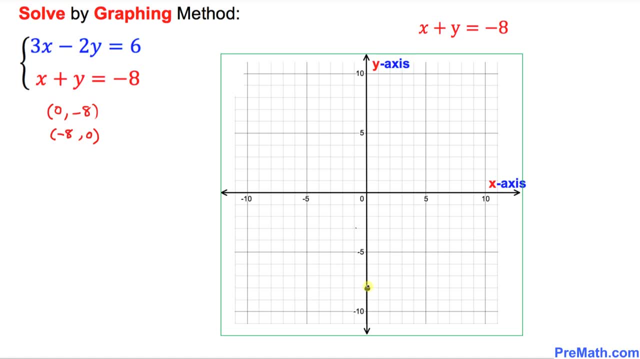 8 is going to be right up here And the other one is negative, 8.. 0 is going to be right up here the point. So once again, this point is on x-axis. We're going to call it x integral. 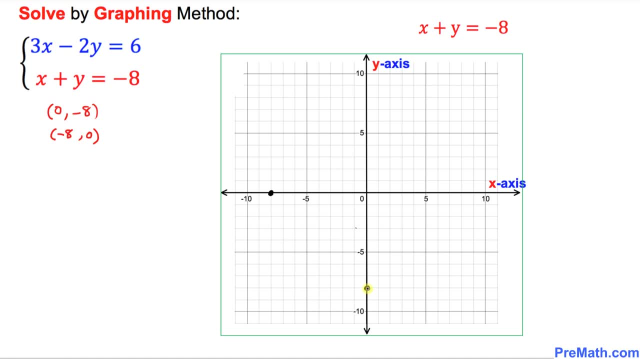 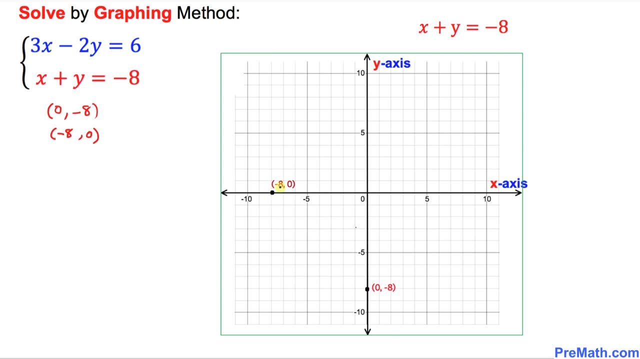 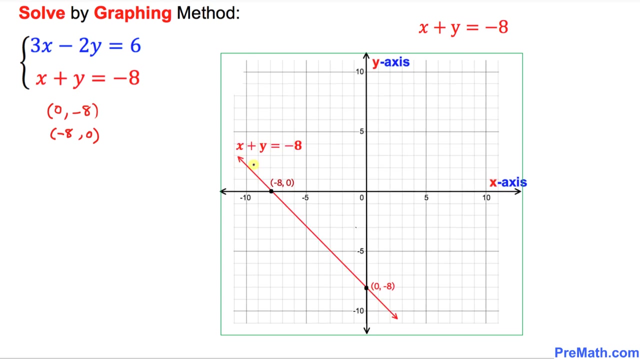 And this point on y-axis is called y intercept. And here I have nicely plotted these points and give them a name: negative 8, 0.. And this is 0 comma, negative 8.. The next step is we are going to connect these two points to get our straight line graph. And finally, here is the graph for x plus y. 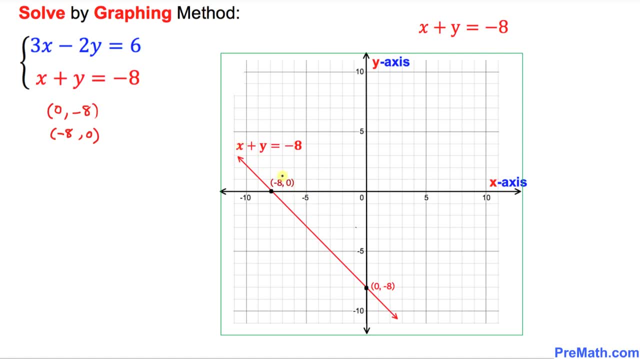 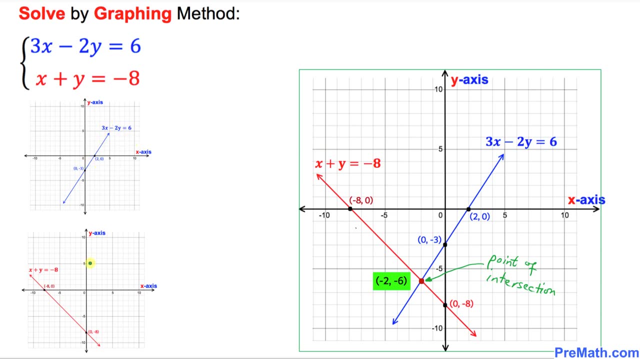 equals to negative 8.. So we are going to connect these two points to get our straight line graph. And here is our final product. And on the left hand side you see these two individual graphs And when I superimpose them I put them together. This is the point. negative 2: negative 6. This is 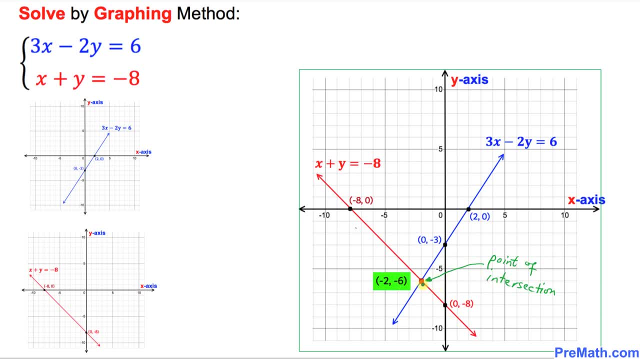 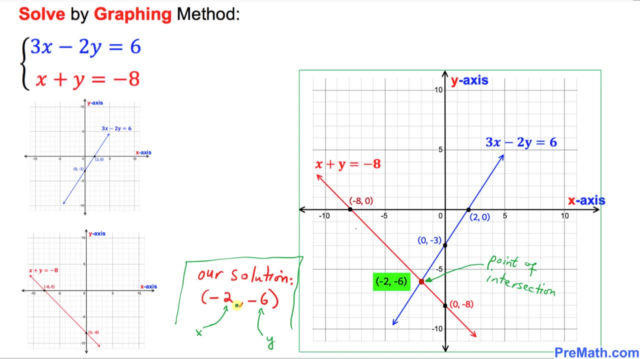 the point of intersection of these two lines, And that is our solution. So thus, our solution turns out to be a negative 2 comma negative 6.. That means x is negative 2 and y is negative 6.. And here is your assignment. Can you do this? 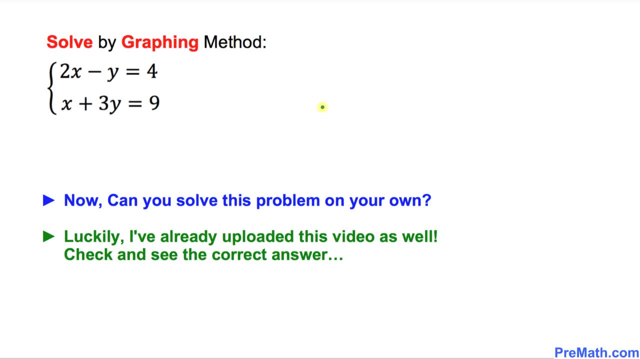 problem on your own. You can take your time. You can pause the video. Luckily, I have already uploaded this video as well. Please go ahead and check it out and see the correct solution. Thanks for watching And please don't forget to subscribe to my channel for more exciting videos. Bye.